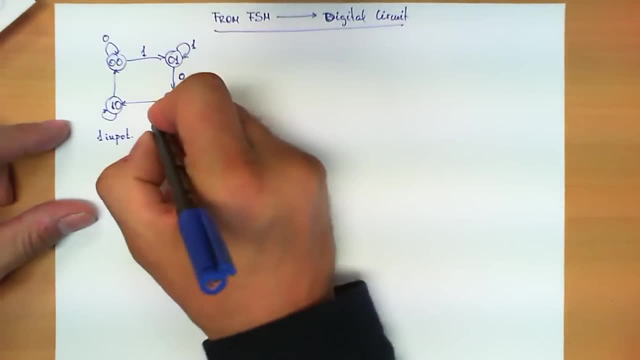 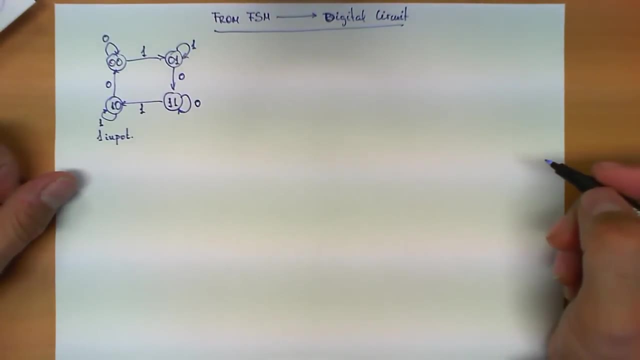 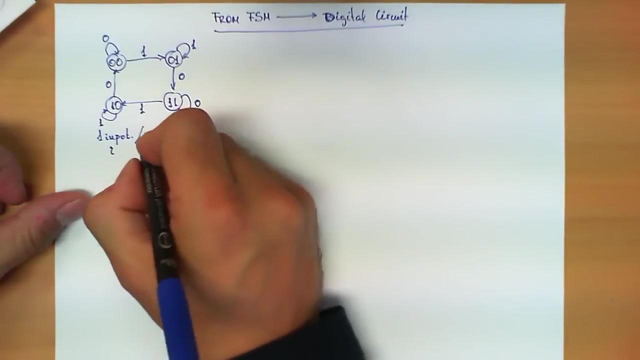 shown here. So this is our starting point: a fully specified finite state machine. Now, aside from one input, which we are going to call I, we also have the state of the finite state machine that we are going to represent with two bits: S0 and S1. 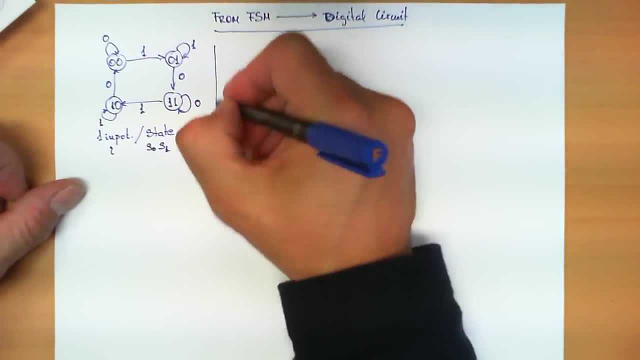 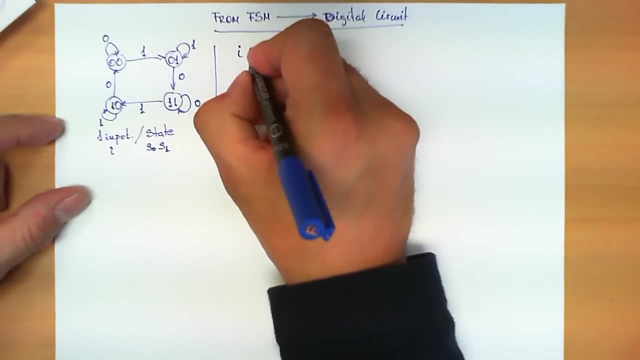 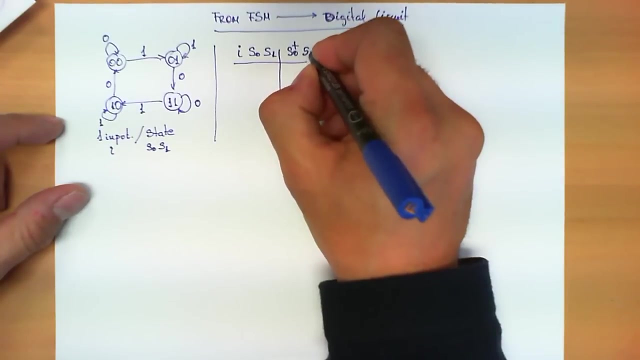 As we can see here, we have two bits. Now. from this description we can derive the truth table in which I, S0, and S1 are used to compute the values S0+ and S1+, denoting the next states to which the machine is making a transition. 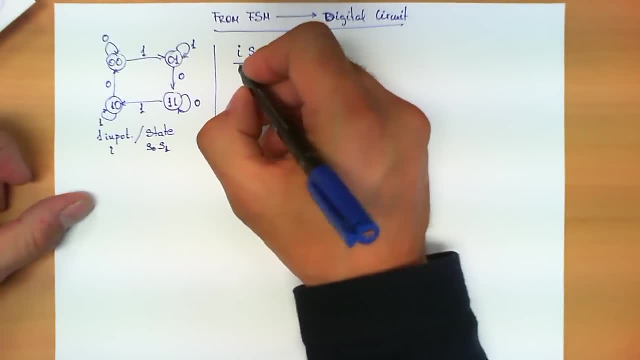 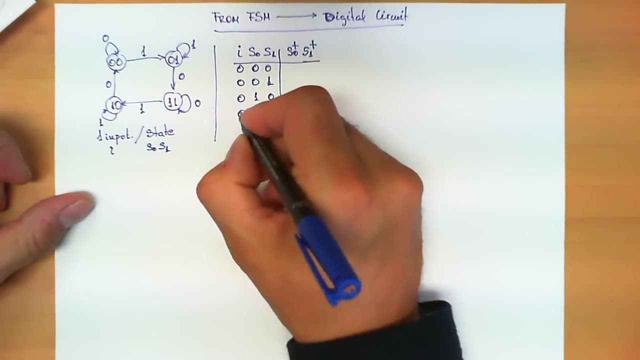 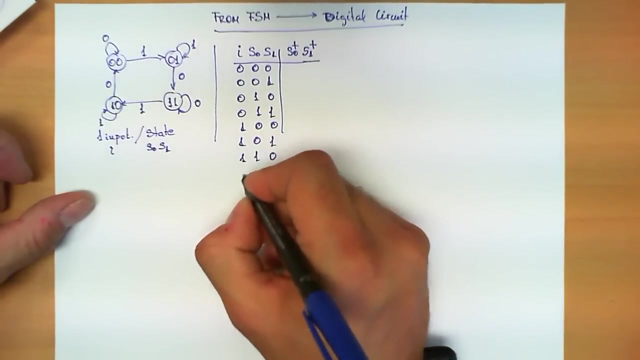 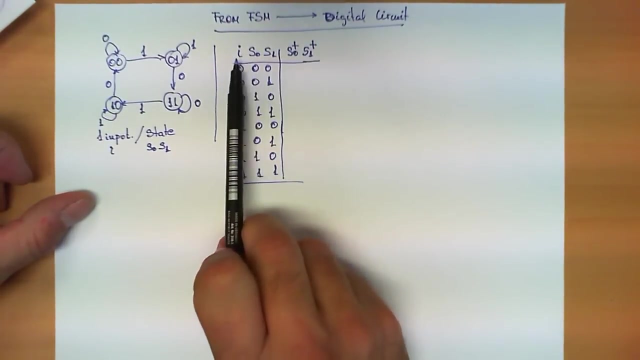 Since we have three Boolean variables here, we need to write eight combinations: 00, 00, 001, 002, 003.. 011, 100, 101, 110, and finally 111.. So these are the eight possible situations when we consider input and current state. 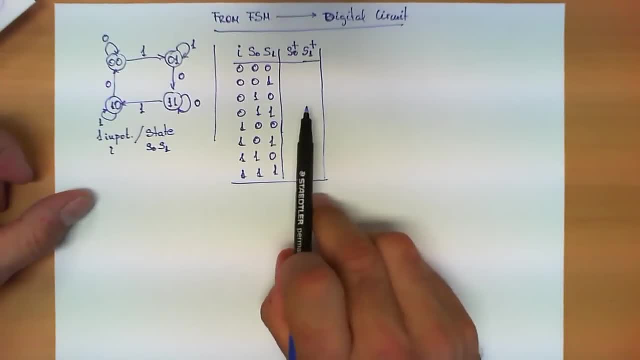 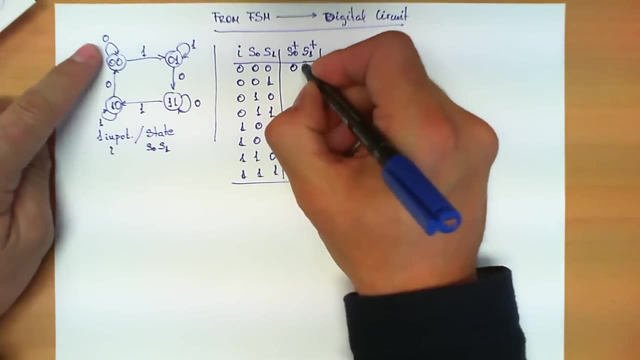 And now we have to derive the values of the next state, And we derive this simply by looking at this diagram, So that from state 00,, when it comes to 0,, we make a transition to the same state. When we are in state 01, and we have a transition 0,, we go to state 11.. 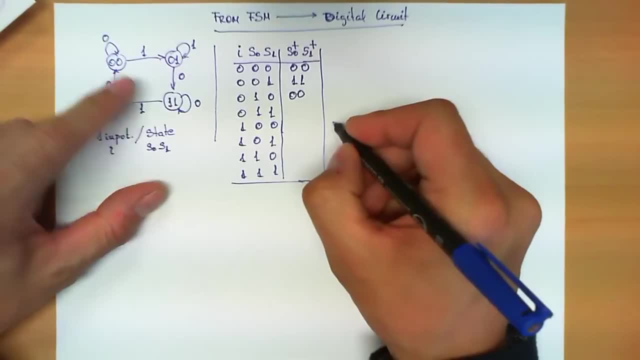 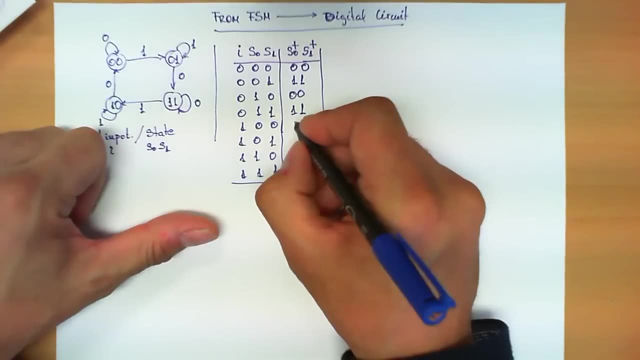 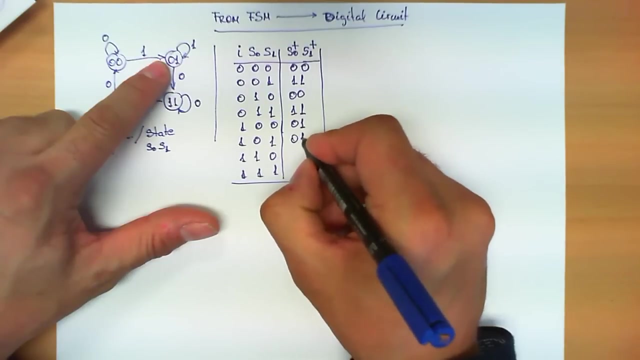 10 with a 0 makes a transition to 00.. 11 with a 0 remains in the same state. 00 with a 1 makes a transition to 01.. 01 with a 1 remains in the same state. 10 with a 1 remains in the same state. 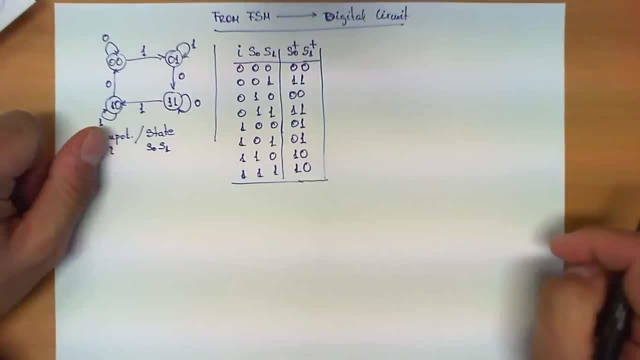 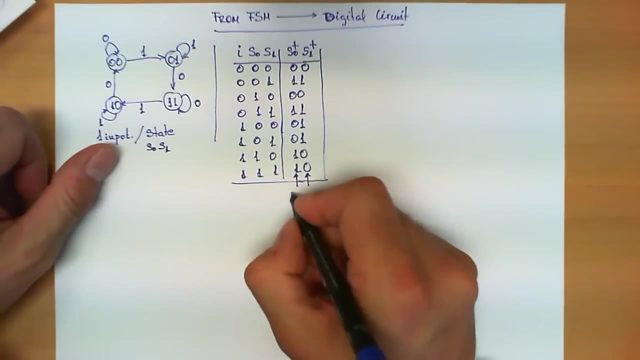 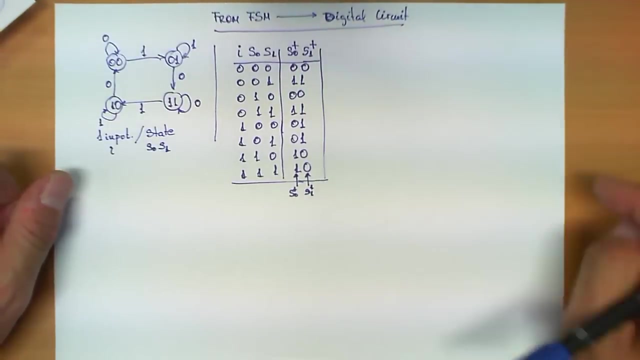 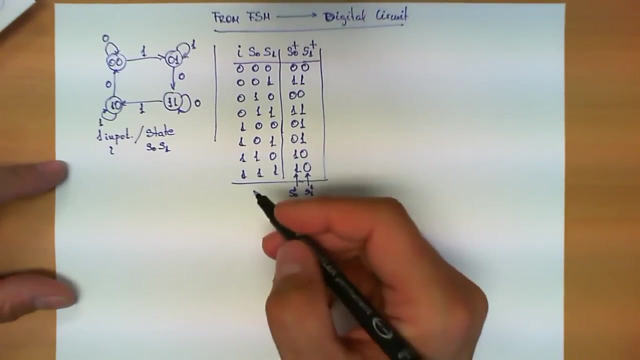 And finally, 11, with a 1 makes a transition to 10.. So what we have here, basically, is the truth table for two Boolean variables: S0+ and S1+. Now the trick to implement a digital circuit from here is simply to implement these two Boolean functions as if they were regular Boolean functions. 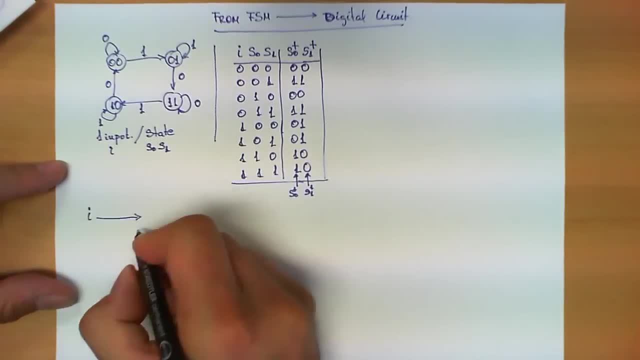 In other words, taking the input i and S0 and S1,, we build a set of logic gates. this will be logic gates that produce as output precisely this column of the truth table S0+, And we're going to have another set of logic gates. 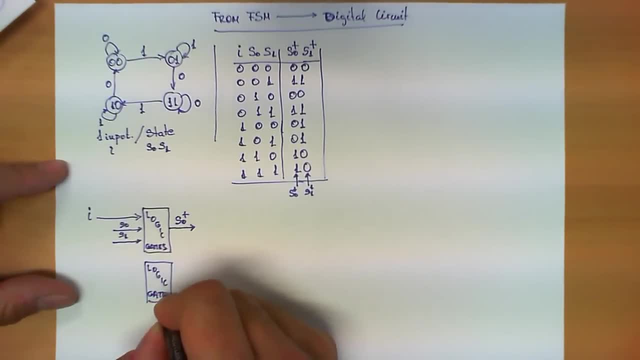 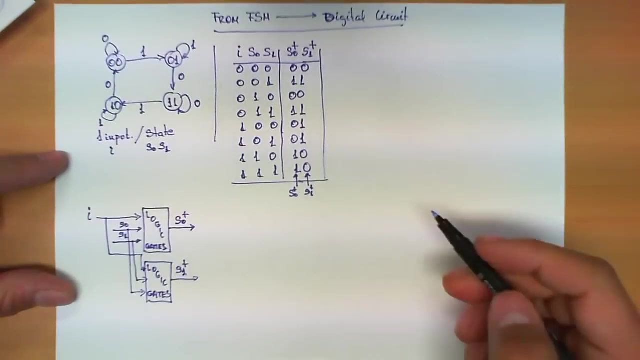 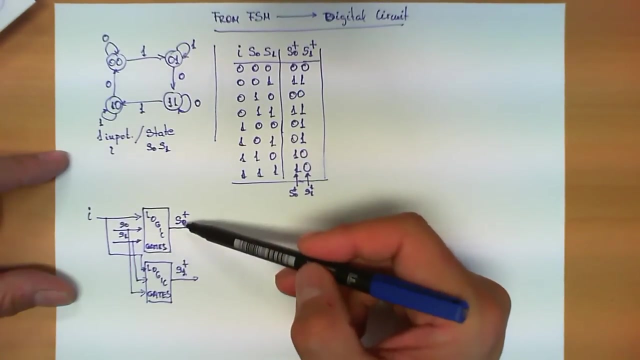 that with the same inputs, in other words the inputs and the state variables, they produce S1+. Now here comes the final touch, to make sure we implement this final state machine, These two variables here, or these two functions. what are telling us is the values that should be the future state. 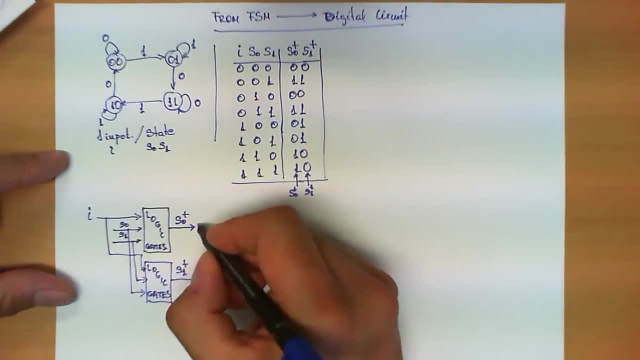 or the state at the next time unit. So these two signals will be stored in a flip-flop, a 2-bit flip-flop, which is going to hold the current state. We can denote this like this with a clock signal. 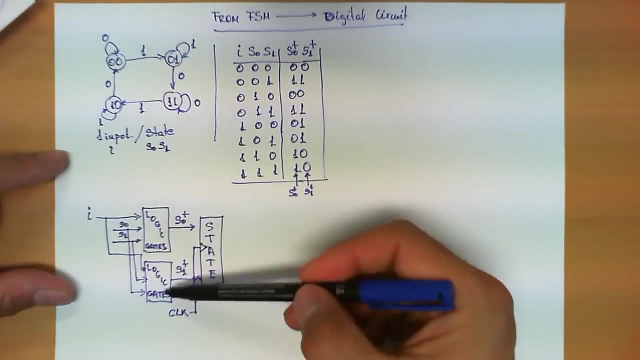 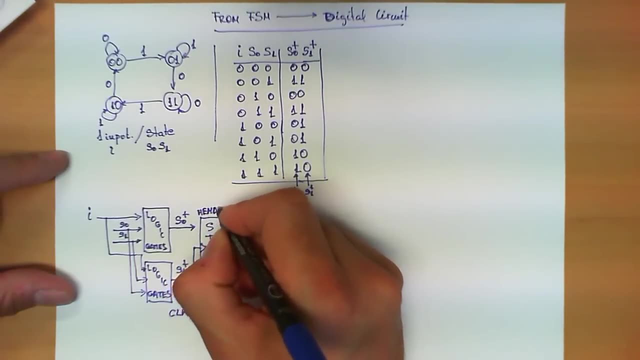 And, as we can see the output of these two logic blocks, it's being now captured and stored. another way of looking at it is that this is an element that has memory and it's captured as the current state of the machine. Now, when the clock signal makes a transition, 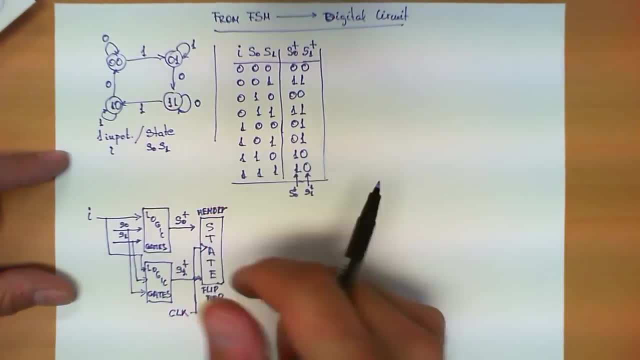 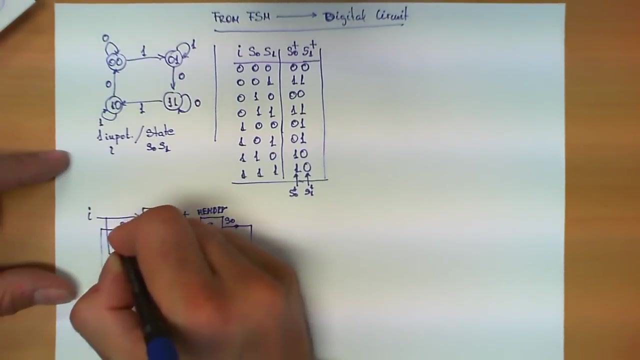 the future state of the machine becomes the current state of the machine, And therefore what we have here is precisely the value of S0.. S1 and S0, and therefore they need to be connected to S1 over here and to S0 over here. 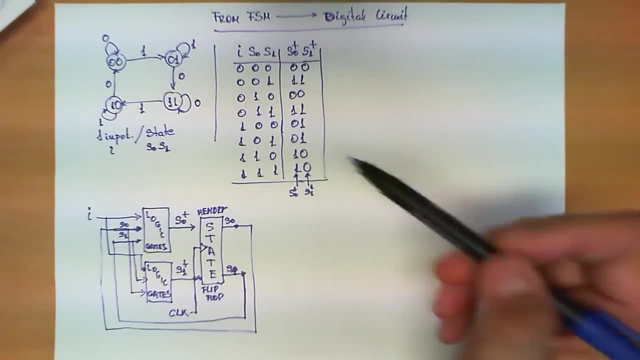 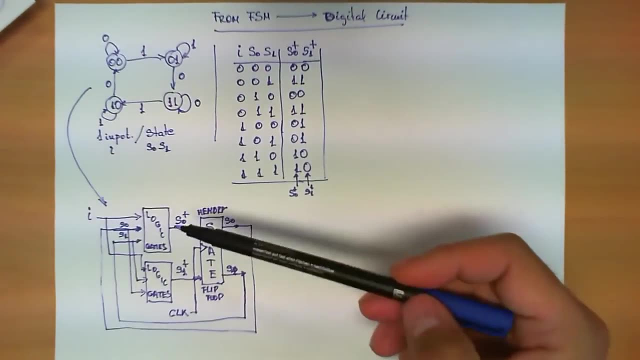 Now this is the resulting implementation of this finite state machine. so we have seen the transition from this diagram to a circuit. but of course we need to implement with gates these two columns over here. Now suppose that we need to implement also some values for certain outputs. 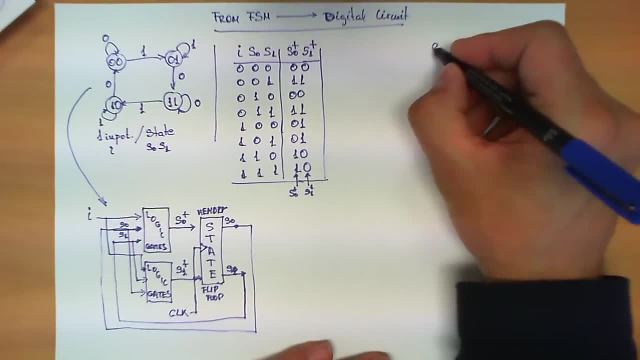 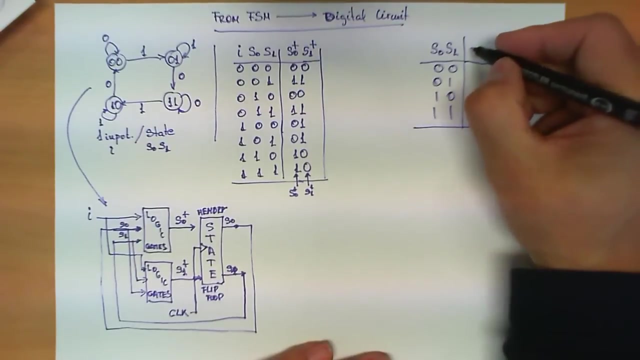 and let's suppose that the outputs of the circuit are only dependent on the state variables. Now we have four states: 00, 01, 10, 11, and let's assume we are extending our finite state machine. let's assume that we have two outputs. 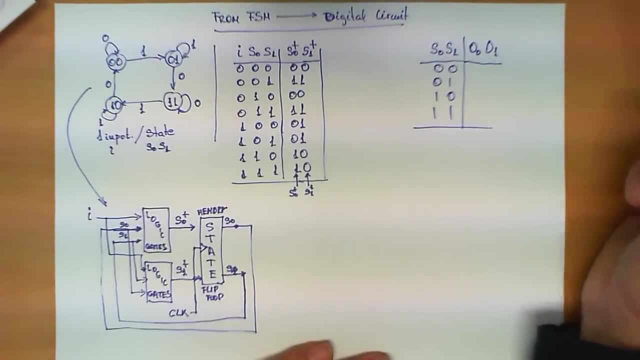 O0 and O1, that depend only on the value of the states. And let's just write some arbitrary logic here. this would be the value of one of the outputs depending on the states, and this would be the value of the other outputs. 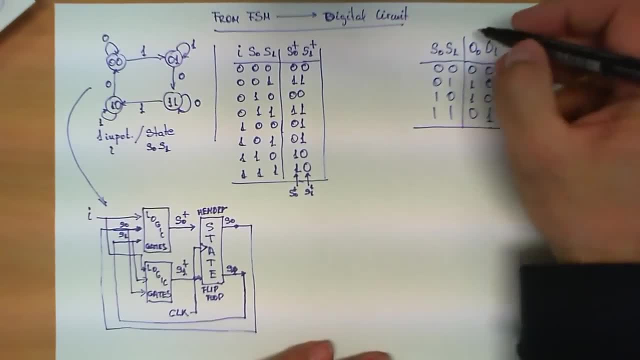 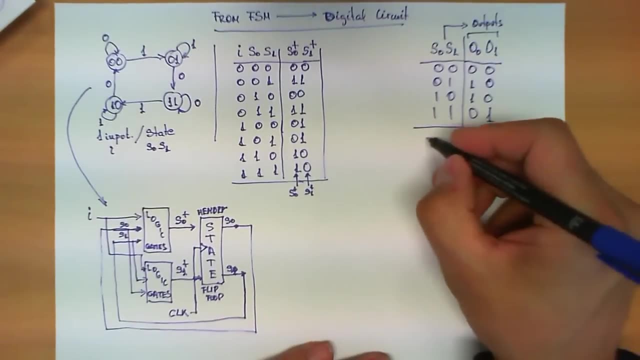 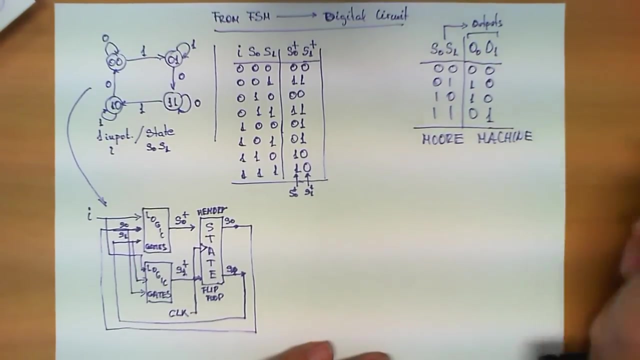 Now one more observation before we proceed. Since the outputs only depend on the value of the current state, this is what is called a Moore machine. How would we implement this? Well, it's very simple. we just need to implement a Boolean function. 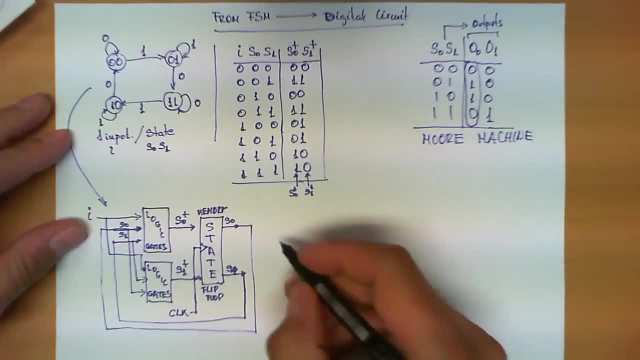 that gives us this truth table, which just so happens to be. if I take this signal- and this signal is actually an XOR gate- this will give me output O0, and in this case, if we look at this truth table, it's actually an AND gate. 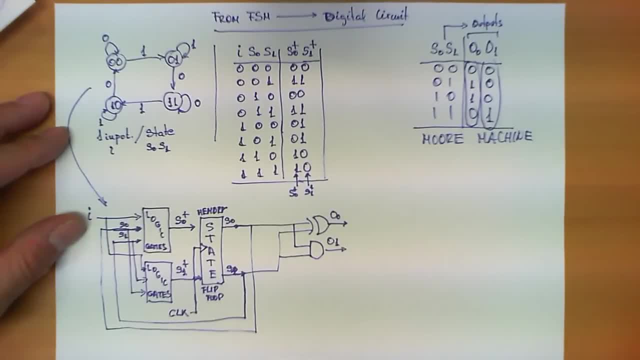 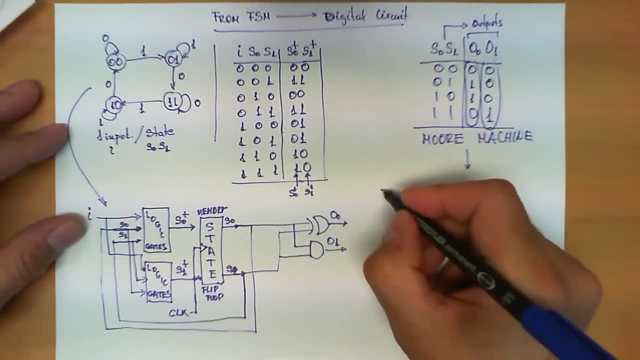 this will give us O1.. So another way of looking at this diagram is the following: In general for a Moore machine, what we're going to have is the inputs going into a set of logic gates and by this box. now I'm lumping together these two. 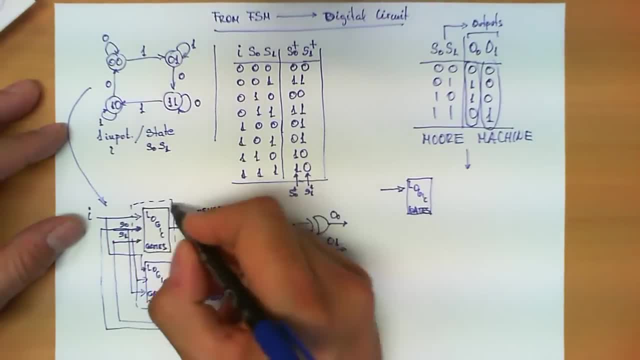 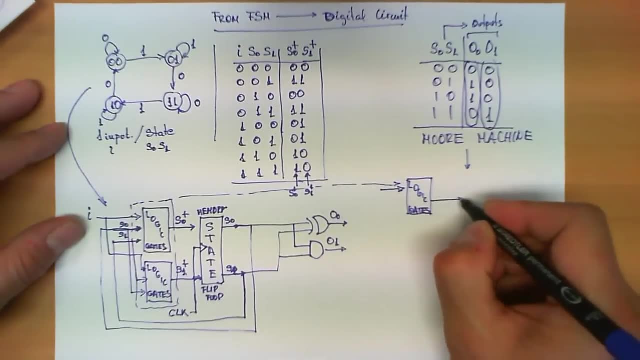 in other words, this would be the block named now logic gates. this block would be in charge of generating all the required signals and signals, whatever is necessary, that feed into a memory element which obviously has a clock which will contain the state. 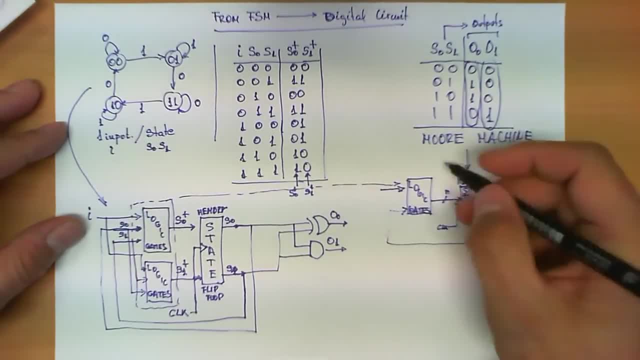 And the value of these variables is also used by these logic gates to compute the next state. Additionally, in case of a Moore machine, there is another block of logic gates here that take the state variables and produce the outputs. So what we have here is 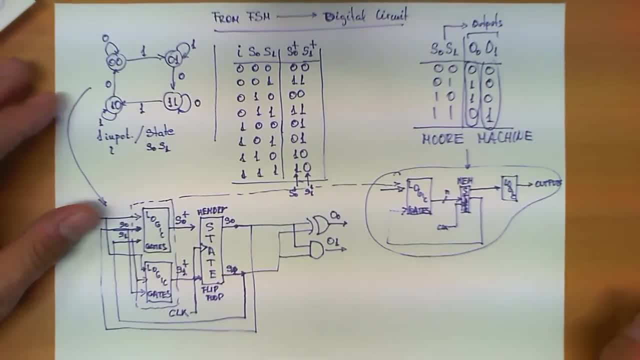 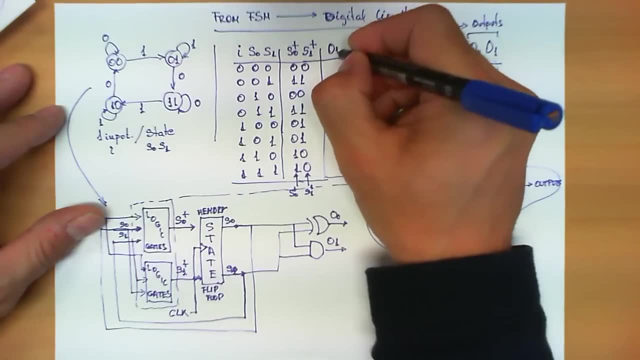 an schematic representation of a Moore machine. Now what happens if what we have is a Millie machine? In the case of a Millie machine, it's very similar. In this case, the outputs O0 and O1 wouldn't depend only on the state variables. 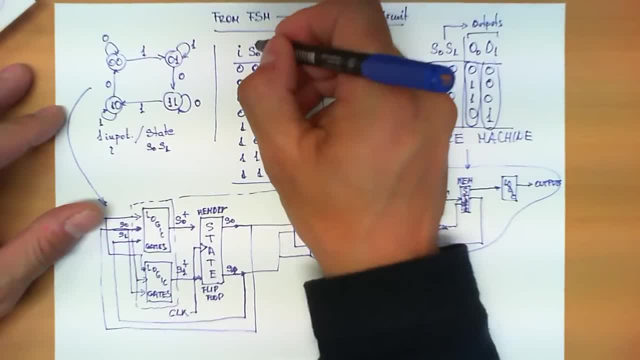 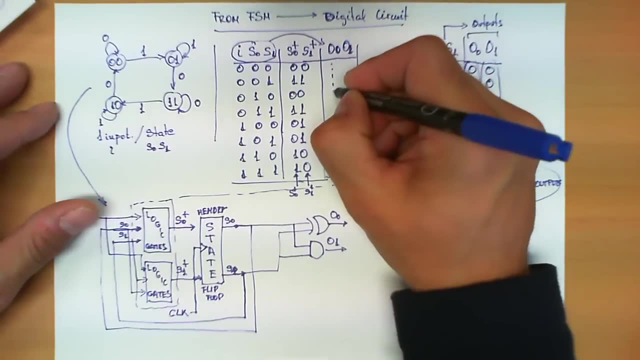 but would depend on the state variables and the inputs. In other words, these three variables will be taken into account to compute the value over here. But again we are in a similar situation. We have two Boolean functions that can be implemented with a set of gates. 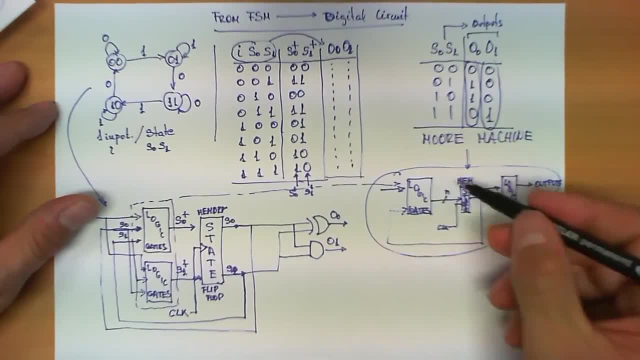 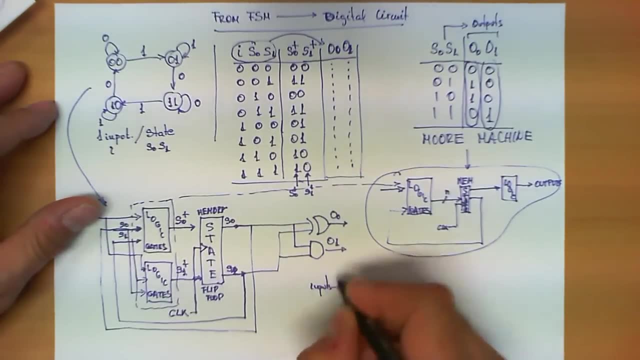 and produce the proper truth table. The equivalent schematic for a Millie machine would be the following: I still have my inputs of the Millie machine. These inputs go into a set of logic gates. These logic gates still produce a set of signals that represent the state.